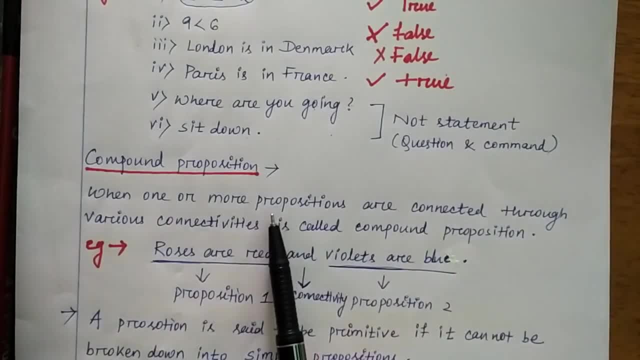 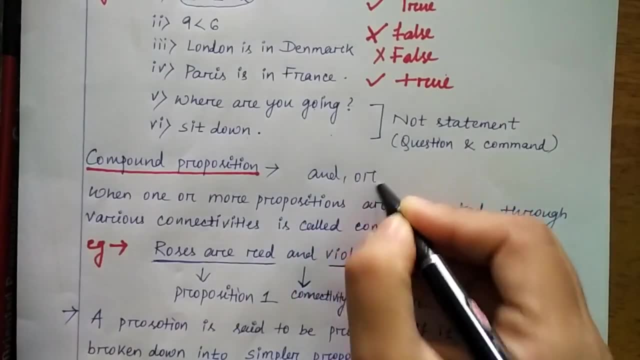 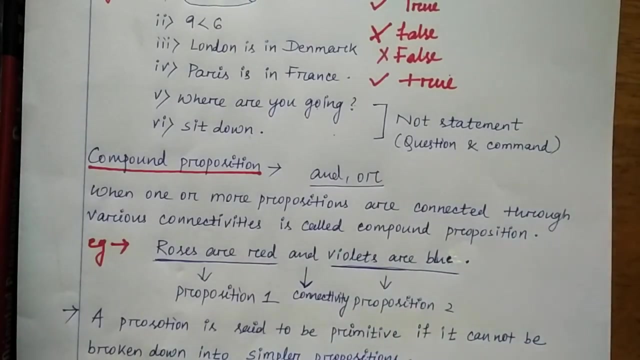 Let me tell you what is connectivity. Connectivity in the sense: how do you join two sentence? Either that can be using a and or by using this two. you can join two sentence: that I am eating my food or I am going to school, or I am eating my food and I am going to school. 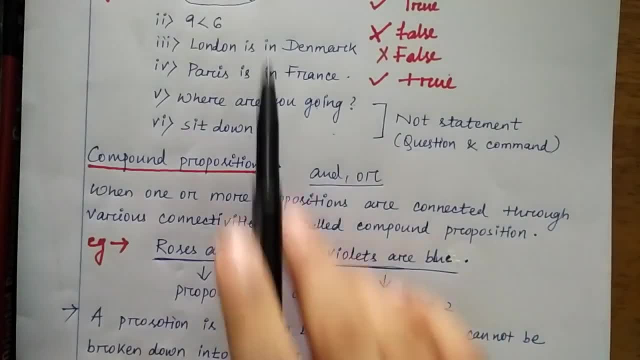 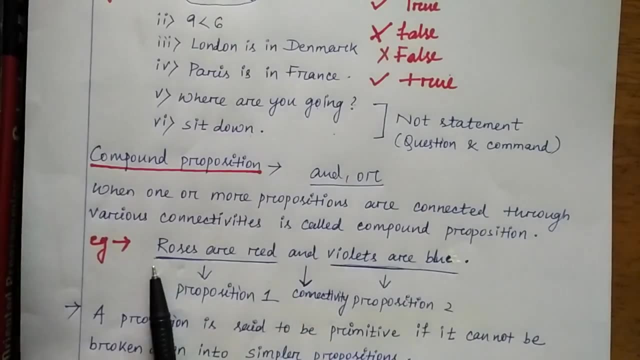 So like that you can connect two different sentence right. The same way when you connect two different proposition to make it as one, that is called as compound proposition. Here we can see an example: roses are red and violets are blue, So roses are red is. 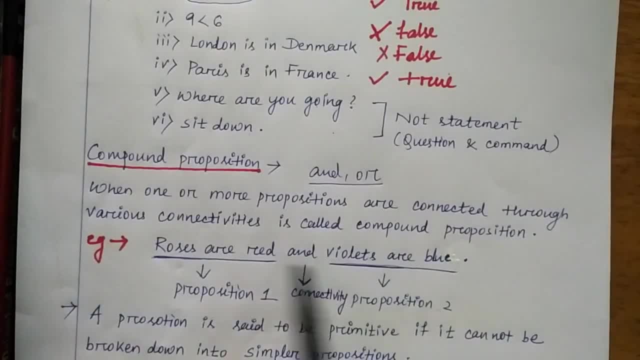 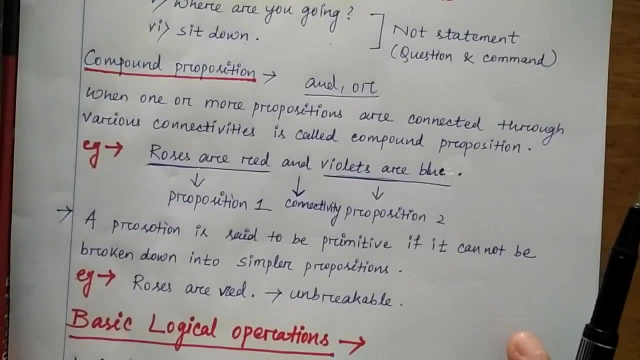 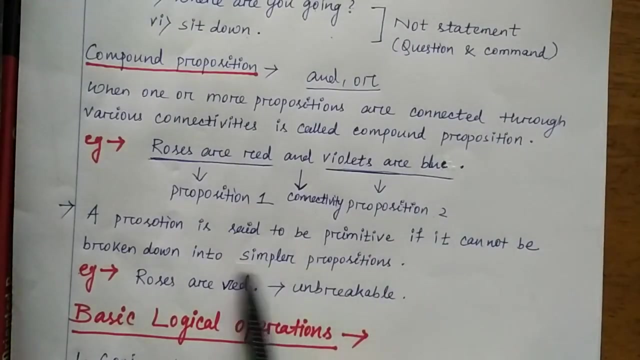 one proposition. violets are blue is the second proposition where we are connecting both of the proposition using the connectivity. and The next point is when you have taken one proposition that is called as primitive one if you cannot break it into simple proposition, Here you have taken a single proposition. 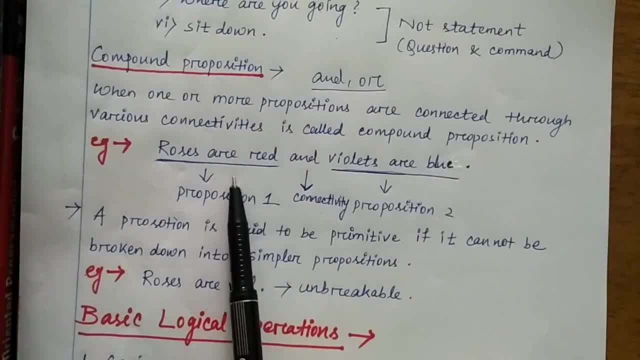 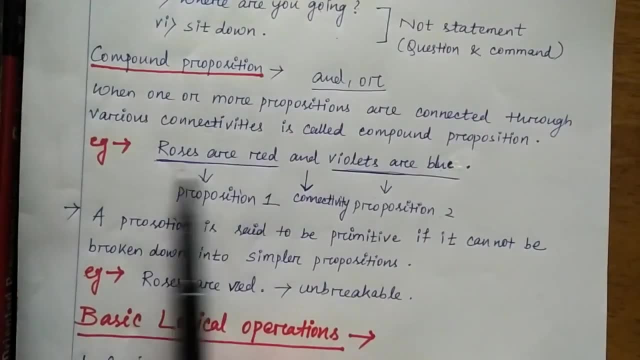 let it be a compound proposition. But you can make it into two different propositions, like roses are red and violets are blue, right. But when you take only roses are red as a proposition, can you break it into two parts? No, right, That cannot be possible. 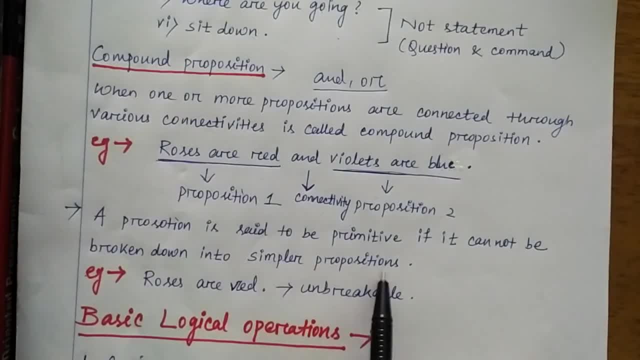 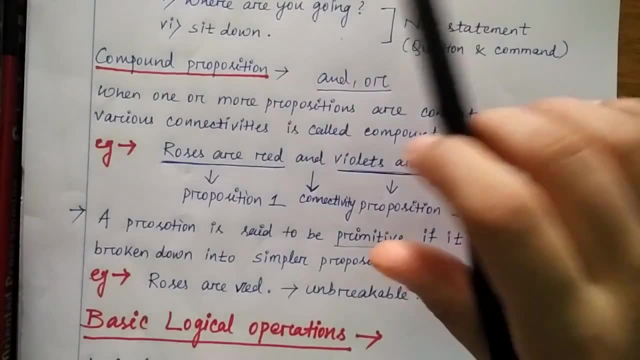 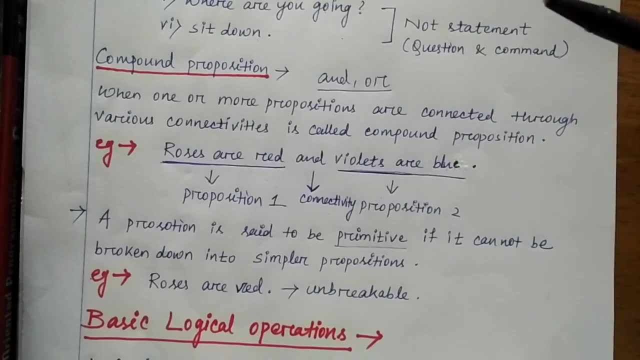 That is why roses are red- is a single, unbreakable proposition which can be called as primitive proposition. So now you are clear. what is a proposition? It is a normal sentence, excluding all that question mark, command statement and exclamatory sentences. 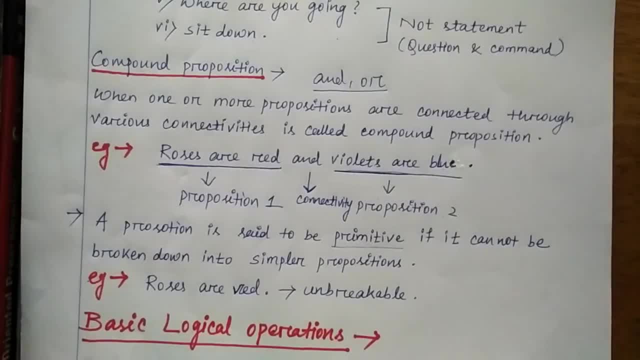 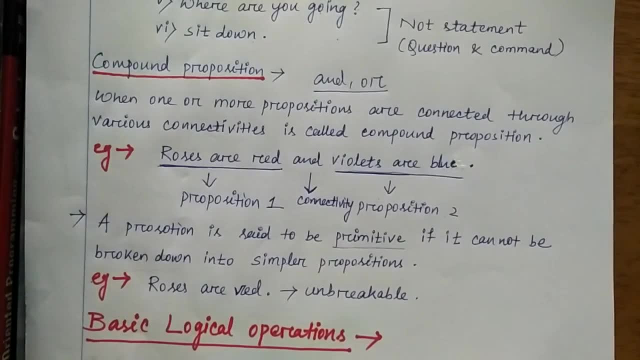 Then compound proposition is when you are connecting two different proposition. And primitive proposition is a single proposition which cannot be broken into many other proposition. But compound can be broken into single two proposition or two or three. That can be up to the number of proposition you are adding into the compound. 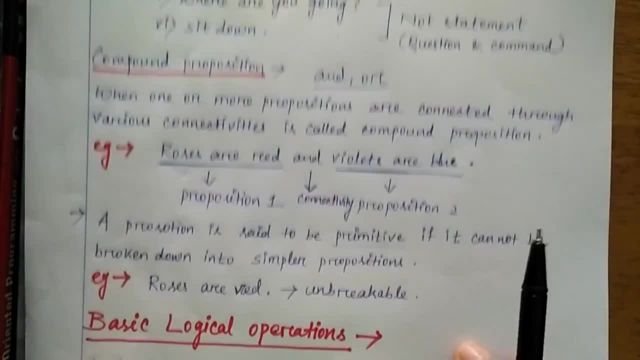 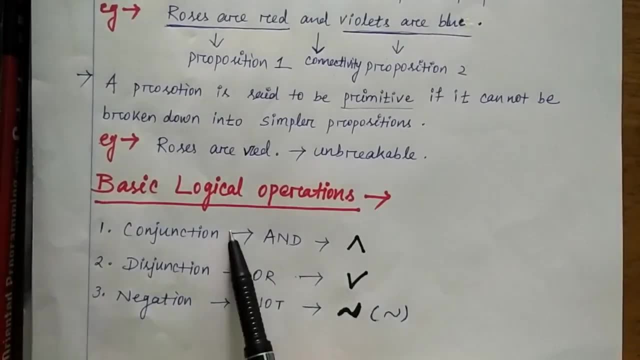 Okay, so next topic is: we will see about the basic logic operation. So basic logic operation are the three types, that is, conjunction, dissection and negation. Actually, logic operation can be of many type, but the basic ones are conjunction, dissection, negation. 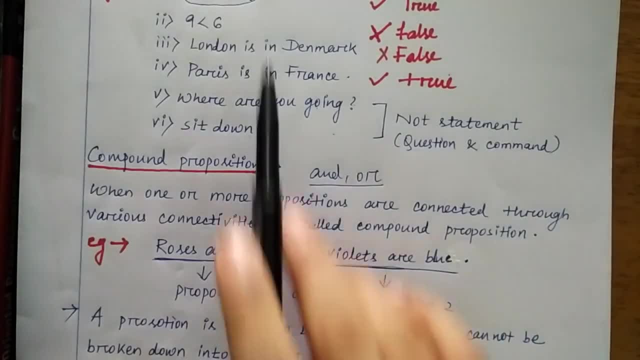 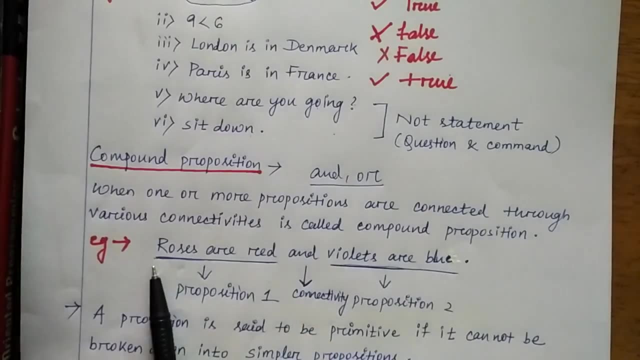 So like that you can connect two different sentence right. The same way when you connect two different proposition to make it as one, that is called as compound proposition. Here we can see the example: roses are red and violets are blue, So roses are red is. 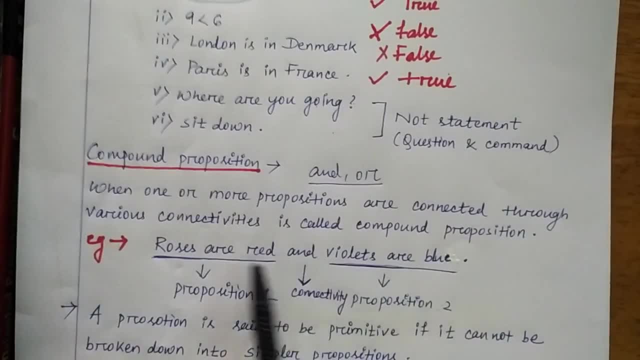 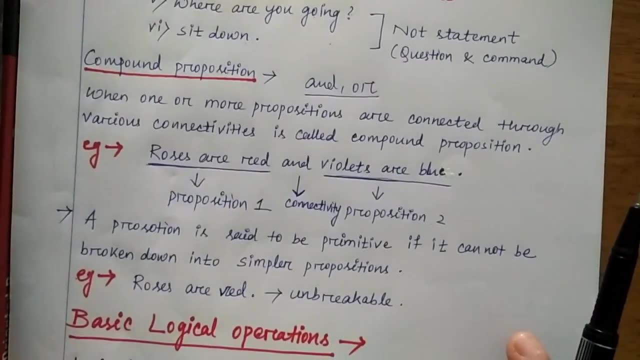 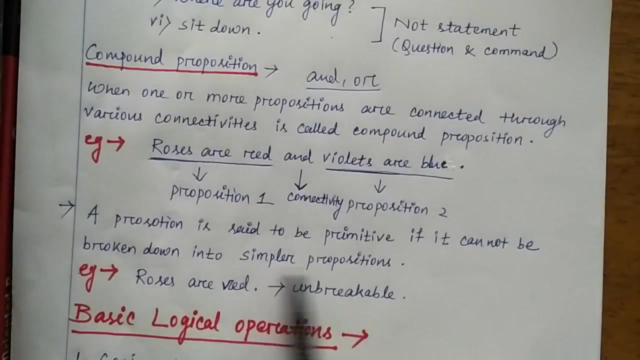 one proposition. violets are blue is the second proposition where we are connecting both of the proposition using the connectivity and. And the next point is when you have taken one proposition that is called as primitive one if you can't break it into simple proposition. 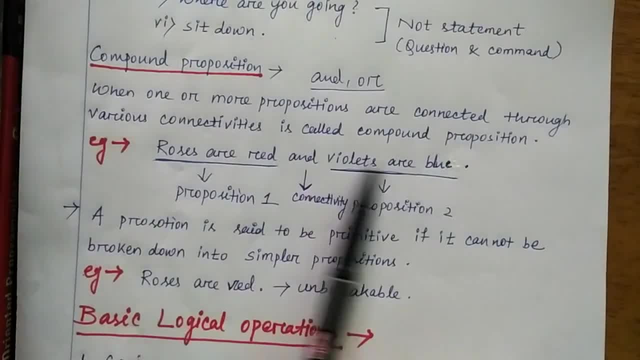 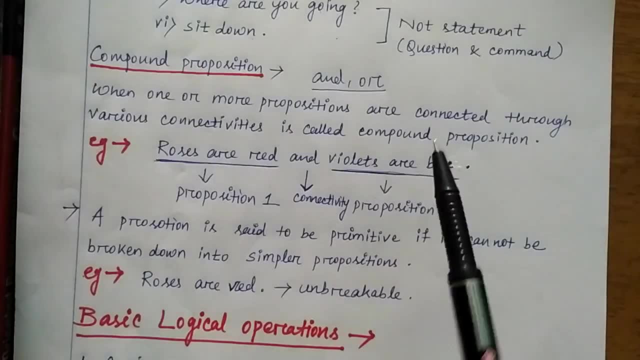 like here: you have taken a single proposition. let it be a compound proposition So you can make it into two different proposition, like roses are red and violets are blue, right, But when you take only roses are red as a proposition, can you break it into two part? 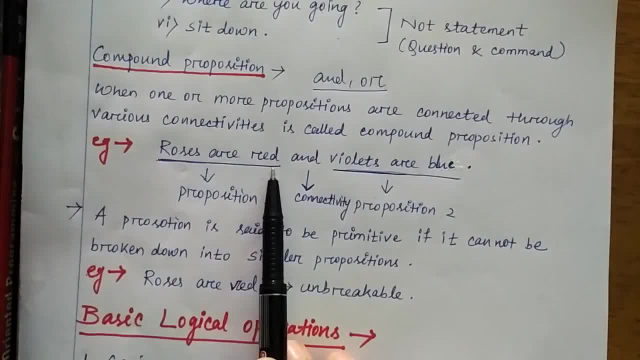 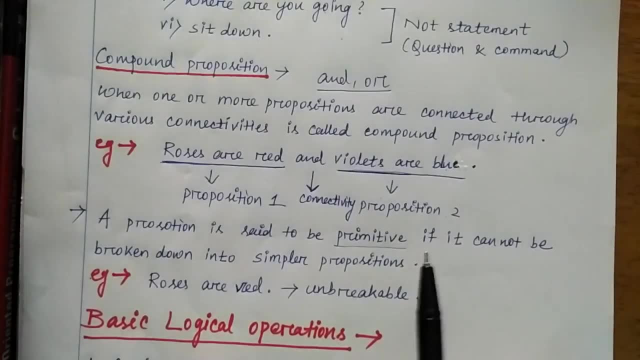 No right, That cannot be possible. That is why roses are red. is a single, unbreakable proposition, which can be called as primitive proposition. So now you are clear. what is a proposition. It is a normal sentence, excluding all that questions, Then mark command, statement and exclamatory sentences, Then compound. proposition is when. 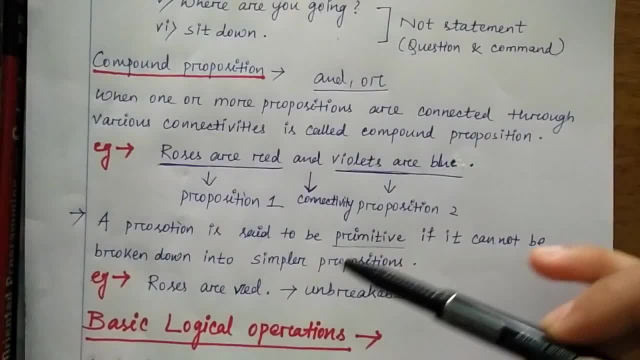 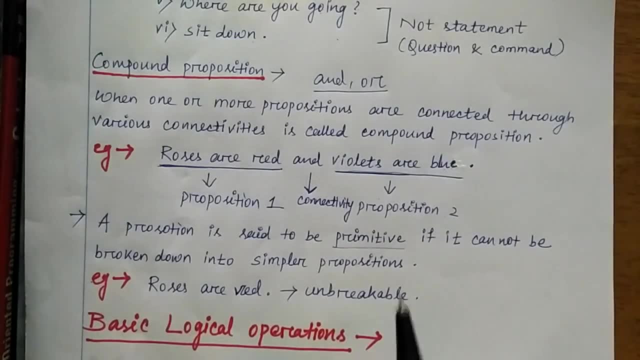 you are connecting two different proposition. and primitive proposition is a single proposition which cannot be broken into many other proposition. But compound can be broken into a single, two, two proposition or two or three. that can be up to the number of proposition you are adding into the compound proposition. 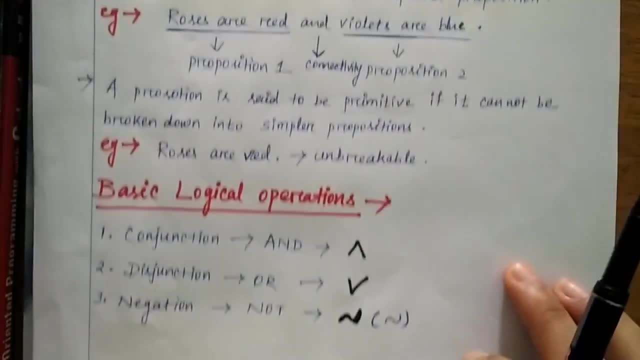 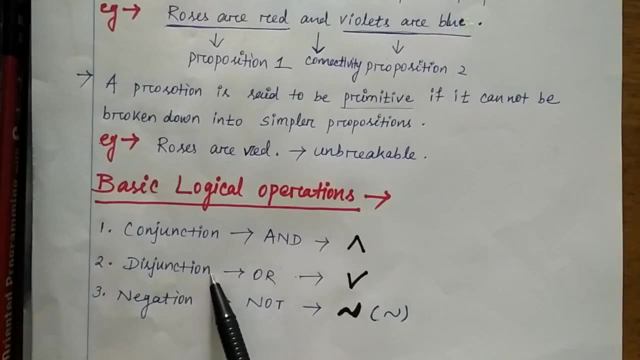 Okay, So next topic is: we will see about the basic logic operation. So basic logic operation are the three types, that is, conjunction, disjunction and negation. Actually, logic operation can be of many type, but the basic ones are conjunction, disjunction, negation, that is, and or not. And conjunction: 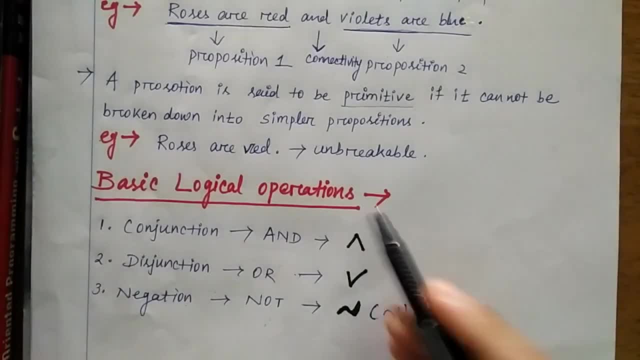 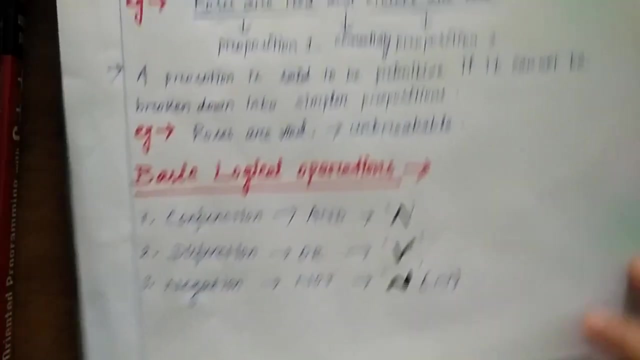 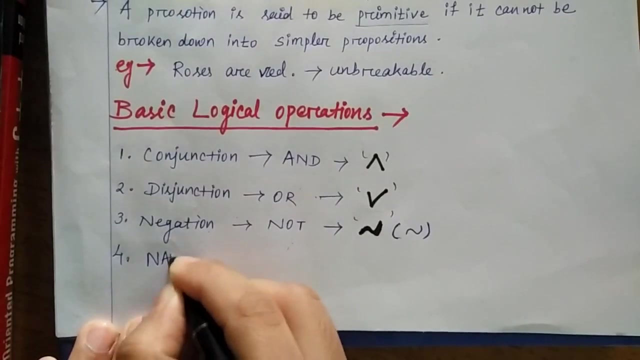 is stand as and in English language, and the notation is this one cap, Disjunction is or The notation is conjunction. The notation is this one: cap and negation is not. The notation is this tilted sign. So I will tell you about the other type of logical operations that can be nand, that is. 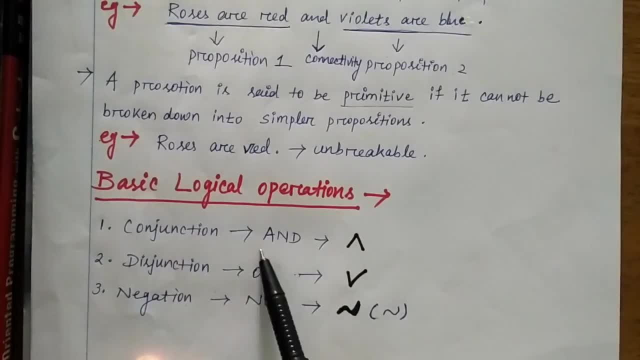 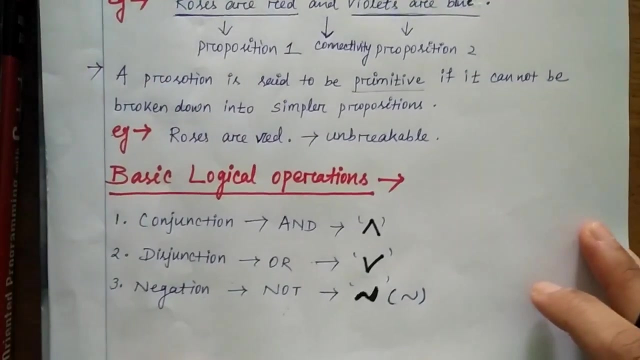 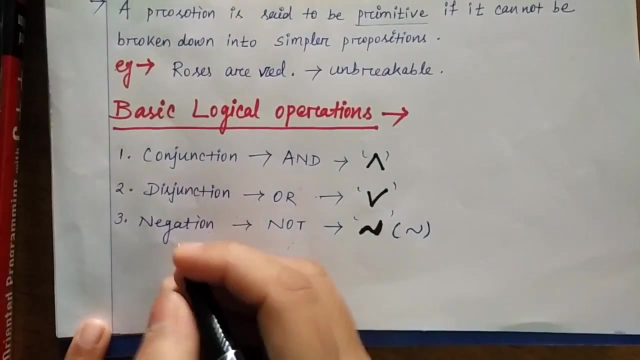 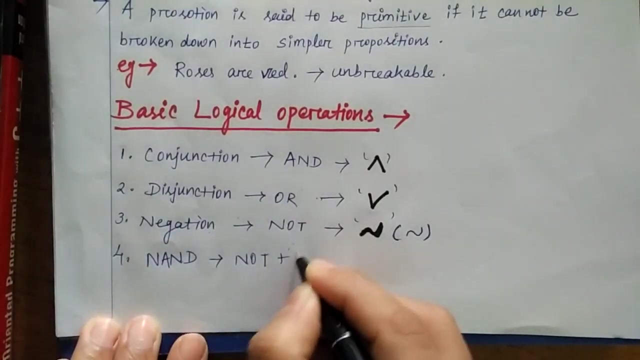 That is and or not, And conjunction is stand as and in English language and the notation is this one: cap. So conjunction is or, the notation is cap, and negation is not. the notation is this tilted sign. So I will tell you about the other type of logical operations that can be nand, that is not plus, and 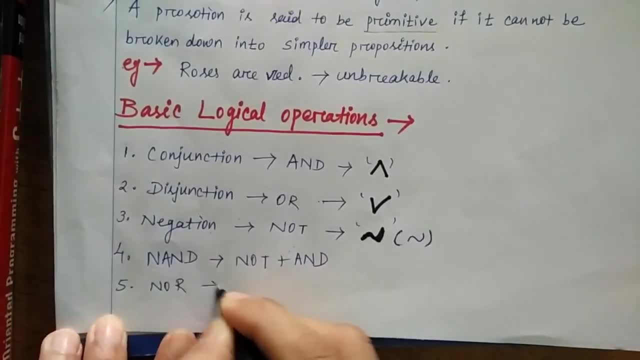 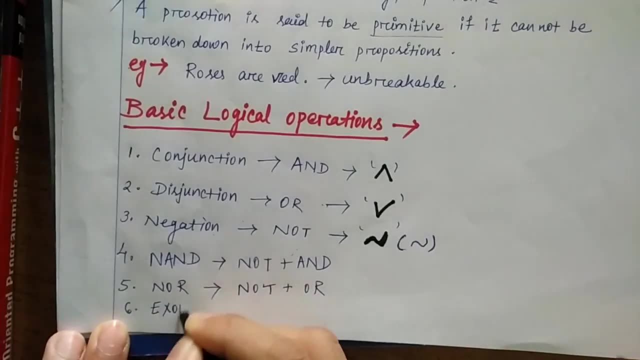 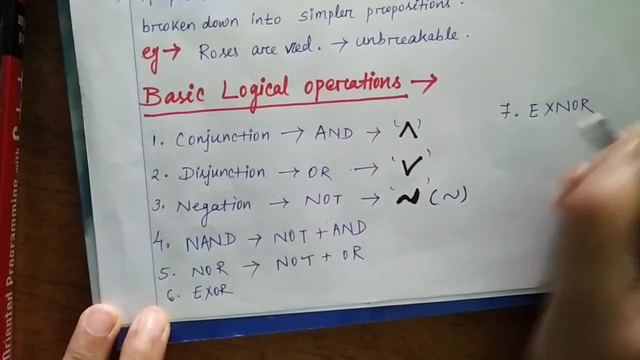 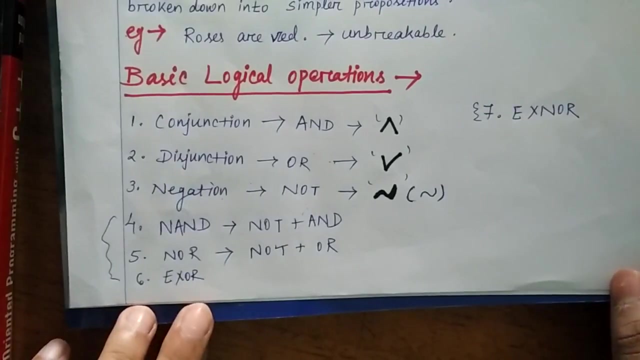 Then next is nor, that is not plus or. And two more are there, that is XOR and next is XNOR. So actually this four we do not use in discrete mathematics but they are there as logic operation in digital electronics. So for timing you should know this three. 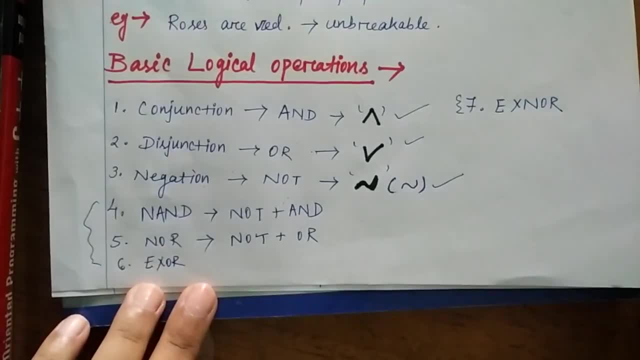 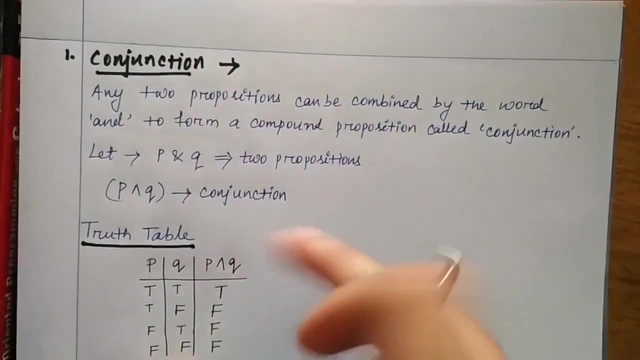 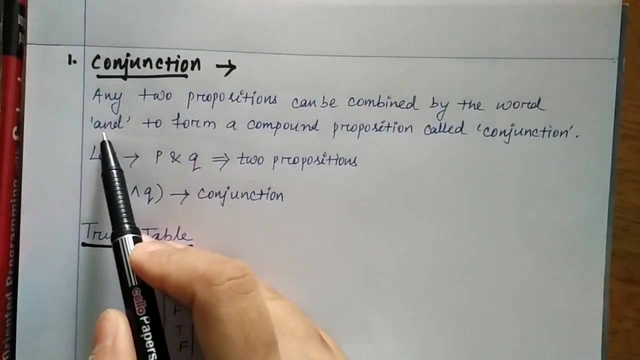 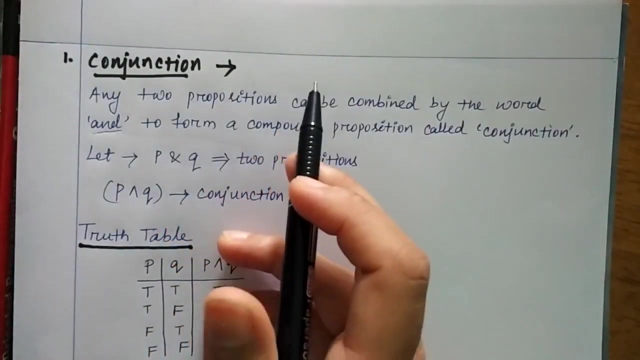 Then we will see what are the truth table of this logic operations. Okay, So the first one we will see: conjunction. Conjunction is when you are adding any two proposition by combining them using the word, and I told you about the connectivity when we considered the compound statement. 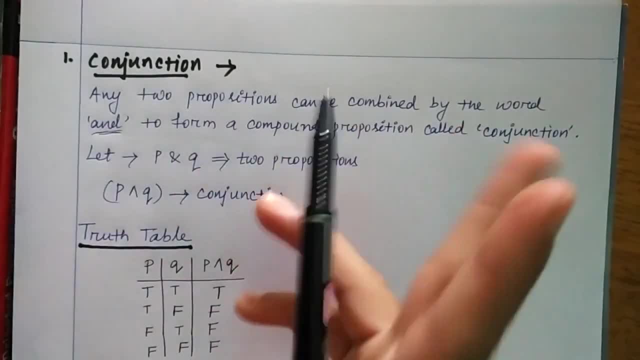 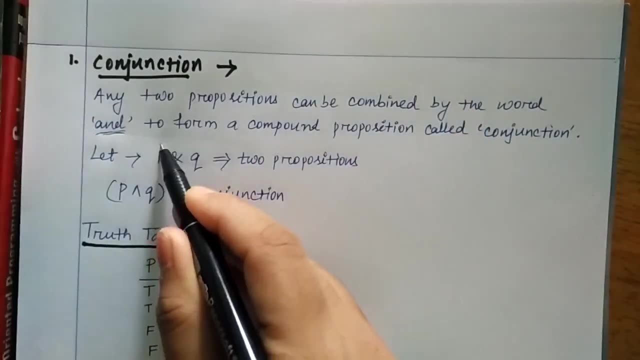 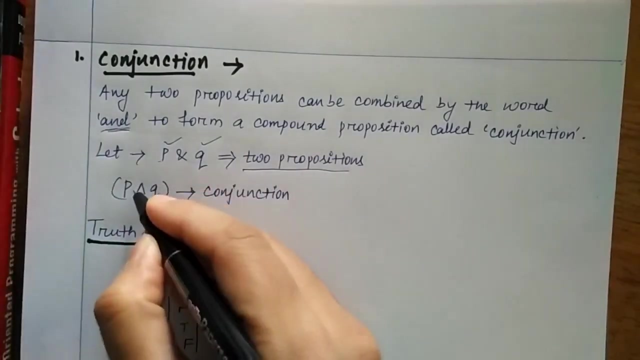 So, in the same way, when you use the connectivity and to connect two different proposition, that is called as conjunction, Instead of taking two different sentence or proposition, I have taken two variables, P and Q, and consider them as two proposition and I have combined them using the operator or using the connectivity and that is the capsimal. 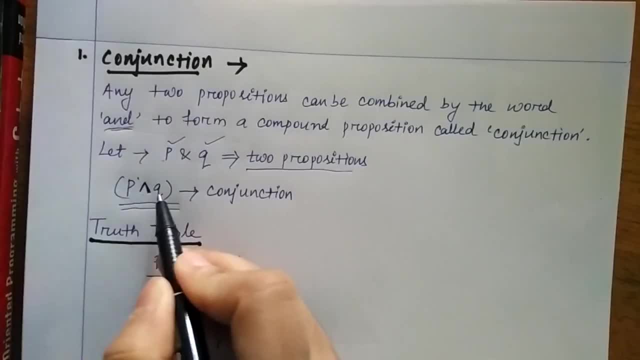 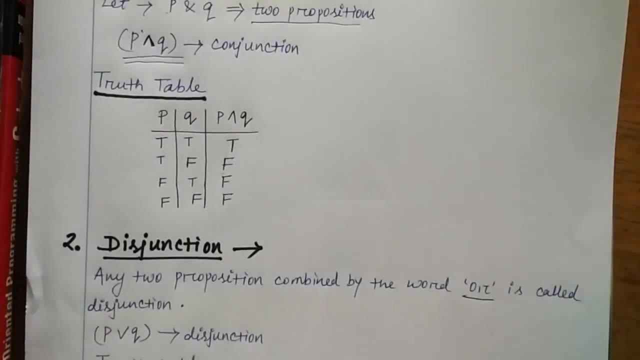 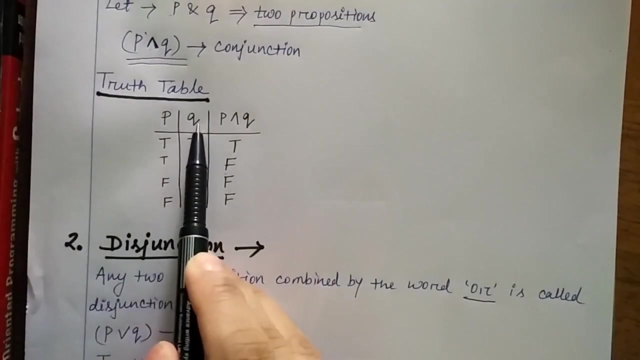 So this is pronounced as, or this is called as, P and Q. Now we will see the truth value. You may ask that why truth table right, I told you that every proposition have a truth value. So see if single proposition have a truth value, true or false for two proposition. 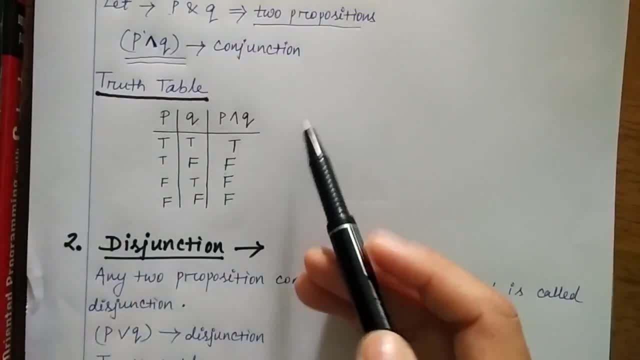 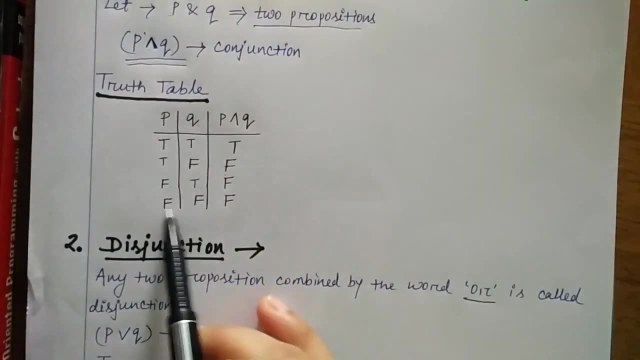 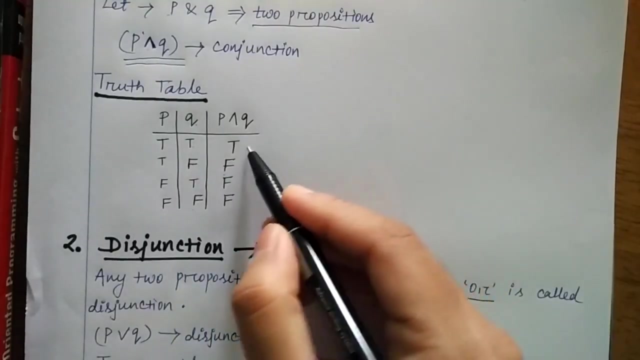 How many truth value you can have four, that is, two cross true, four. then we will see what is the truth table P and Q. if you are taking that is true, true, true, false, false, true and false, false- You are getting four combination of truth values and when you see the result, for true, true, the truth table value always gives the value true and for other value it is false. 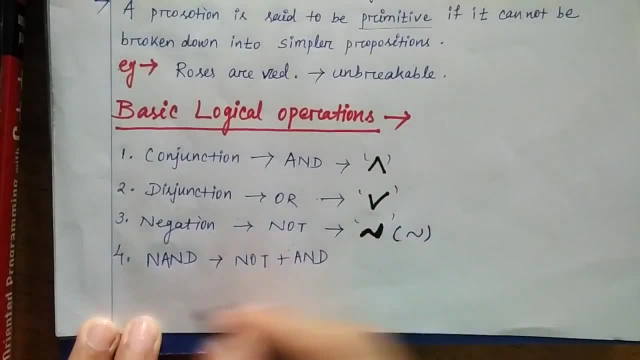 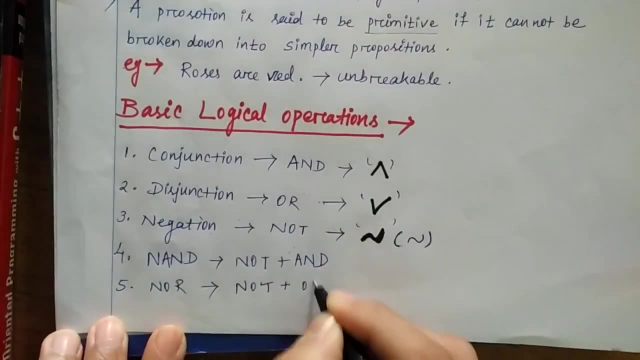 not plus, and Then next is: nor, that is not plus, or, And two more are there. So we will see about the basic logic operation. Okay, So we will see about the basic logic operation. Okay, So we will see about the basic logic operation. 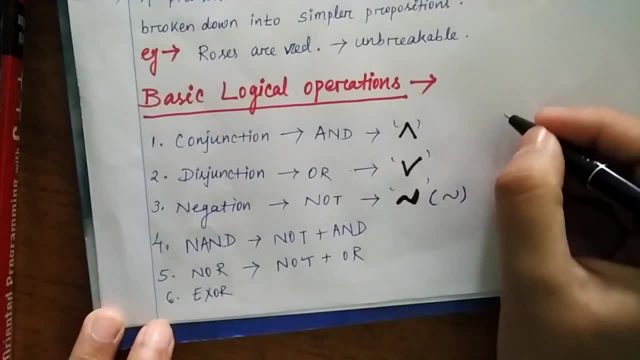 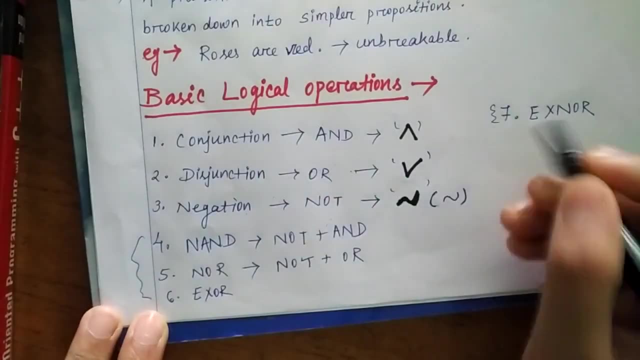 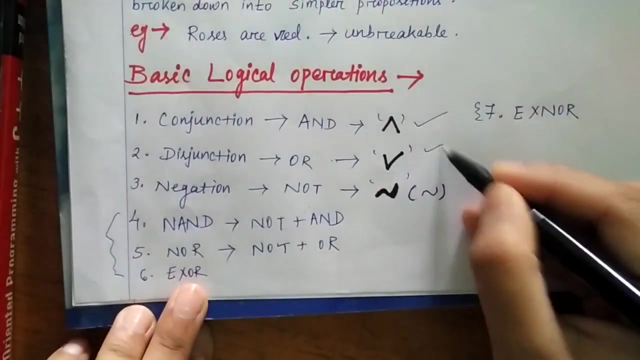 Okay, That is xor. Okay, And next is xnor, Okay. So actually this four we do not use in discrete mathematics, but they are there as logic operation in digital electronic. So for timing you should know this three, Then we will see what are. 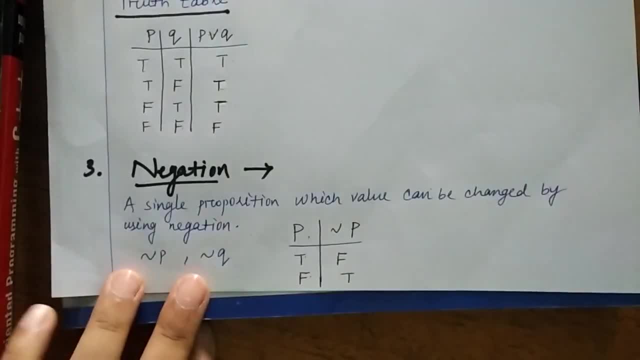 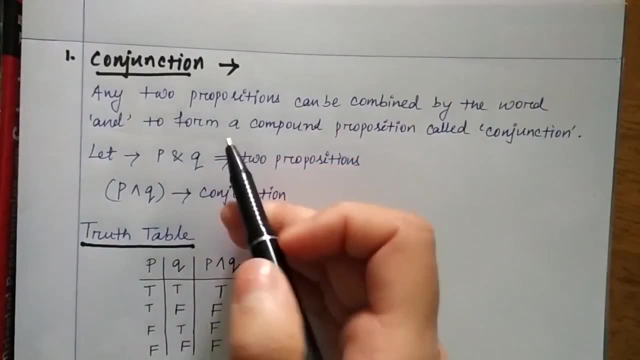 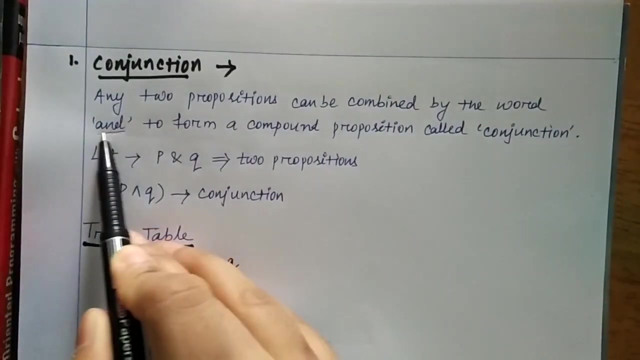 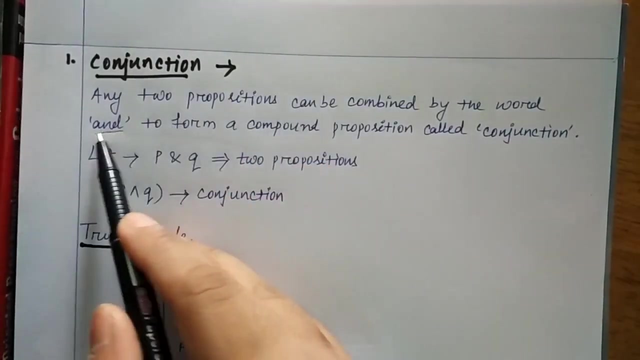 the truth table of this logic operations. Okay, Okay, Okay, Okay, one will see conjunction. conjunction is when you are adding any two proposition by combining them, using the word, and I told you about the connectivity when we consider the compound statement. so, in the same way, when you use the 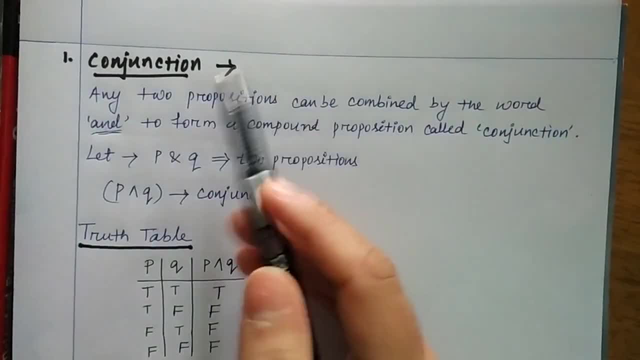 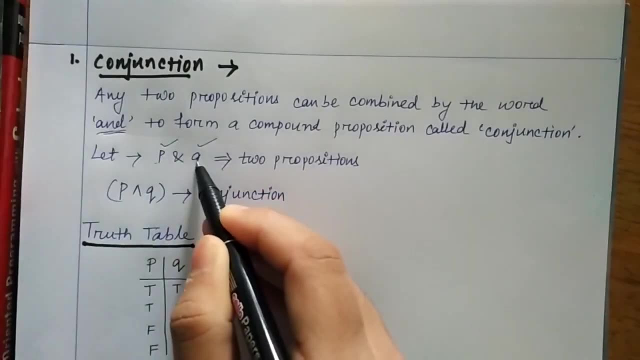 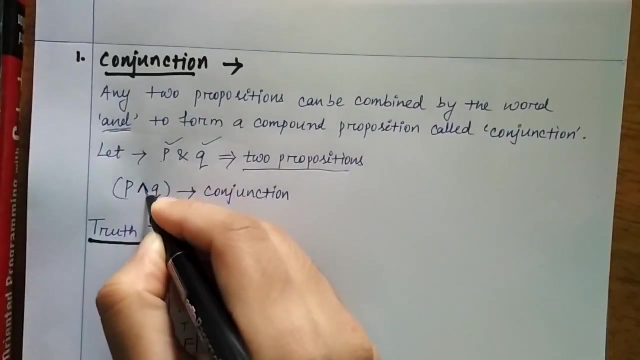 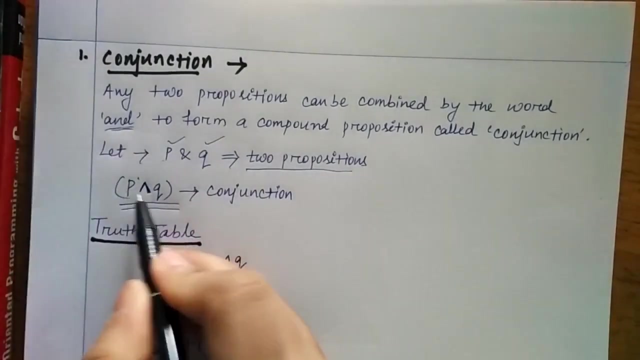 connectivity end to connect two different proposition. that is called as conjunction. instead of taking two different sentence or proposition, I have taken two variable, P and Q, and consider them as two proposition and I have combined them using the operator or using the connectivity end. that is the capsimal. so this is pronounced as, or this is called as, P and Q. now we'll see. 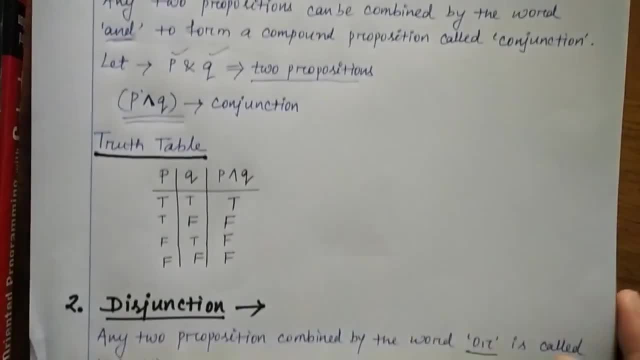 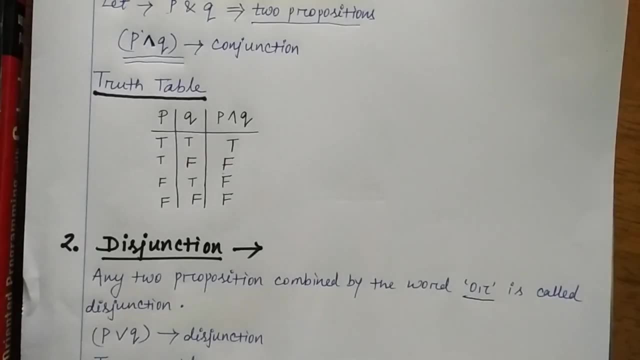 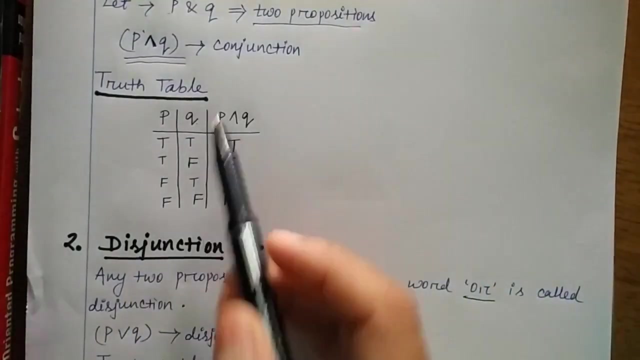 the truth value. you may ask that why truth table? right, I told you that every proposition have a truth value. so see if single proposition have a truth value, true or false. for two proposition, how many truth value you can have four, that is 2 cross true four. then we'll see what is the truth table. P and Q, if you are taking 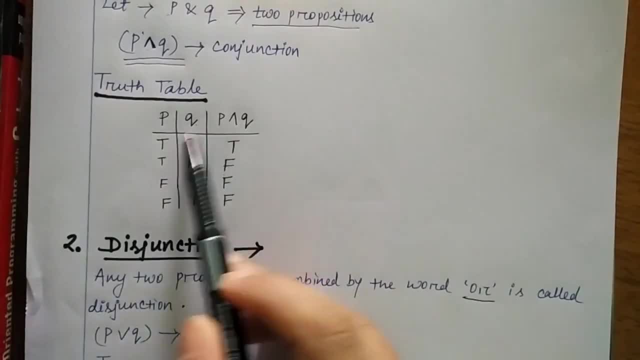 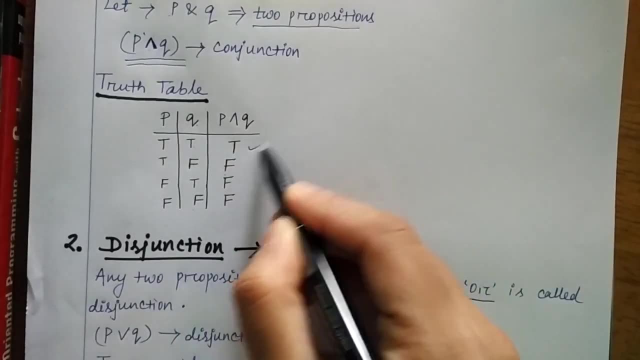 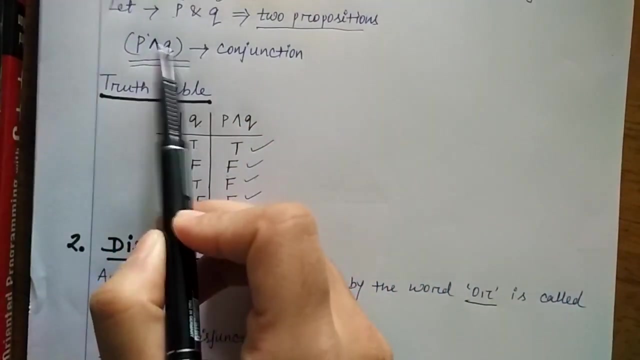 that is true, true, true, false, false, true and false, false, false. you are getting for combination of truth values and when you see the result for true, true, the truth table value always gives the value true and for other value it is false. why true? because when you connect two different proposition using and a 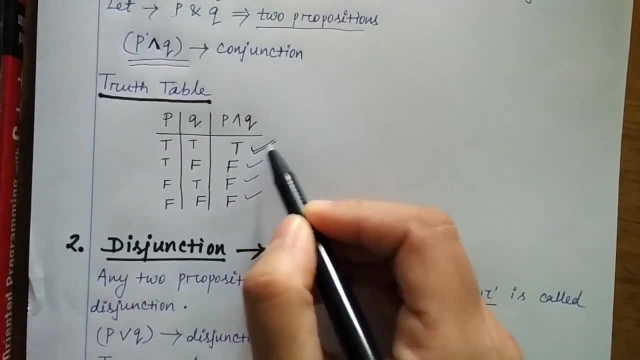 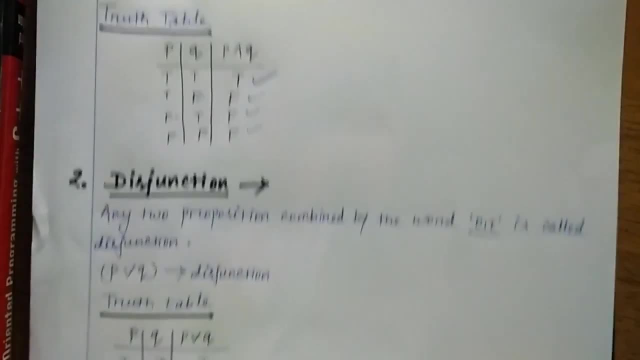 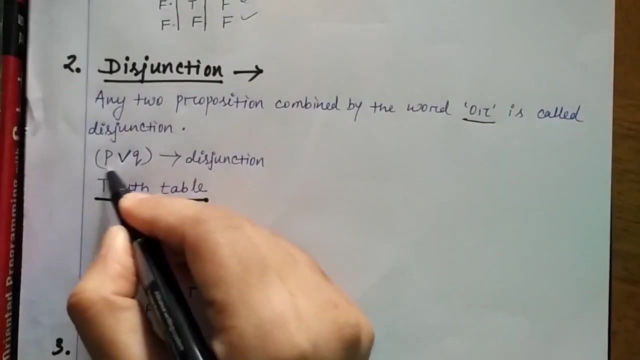 or connectivity, the result is always true. But if any of them is false, or both are false, you will get the result as false. The next is disjunction. Disjunction is when you combine the two propositions using the keyword or, and this is denoted as P or Q, You can see the truth table. First one is true.